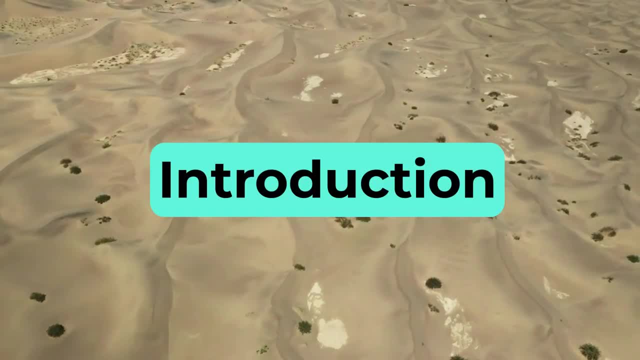 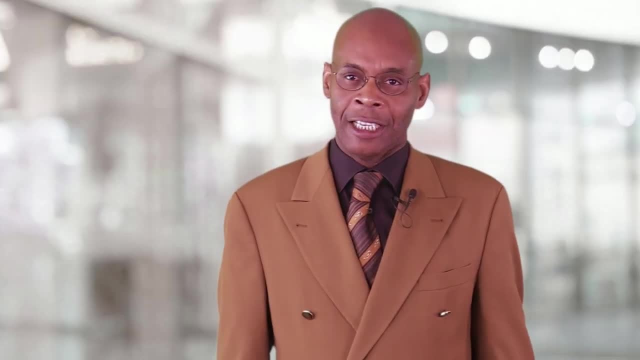 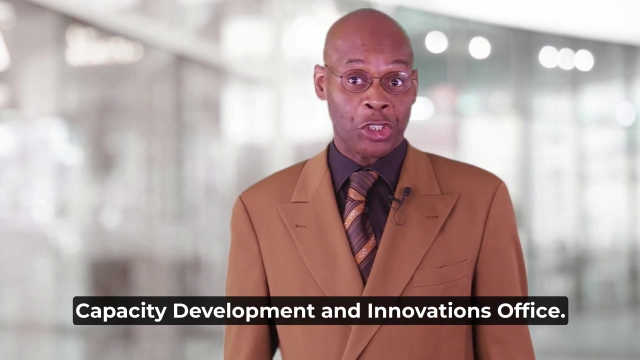 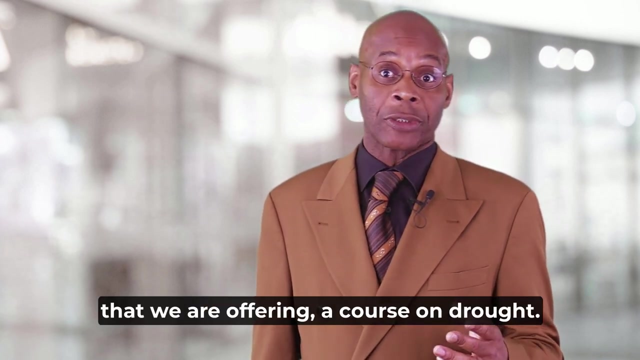 Hello, good day. My name is Richard Byron Cox and I'm head of the UNCCD's Capacity Development and Innovations Office, And today I'm here to introduce you to a new course that we are offering, a course on drought. But before I get to that, you might be wondering what. 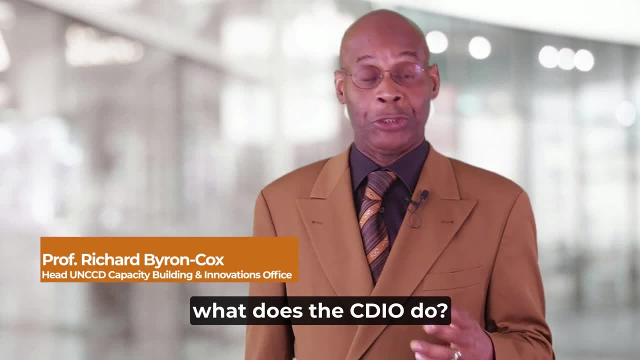 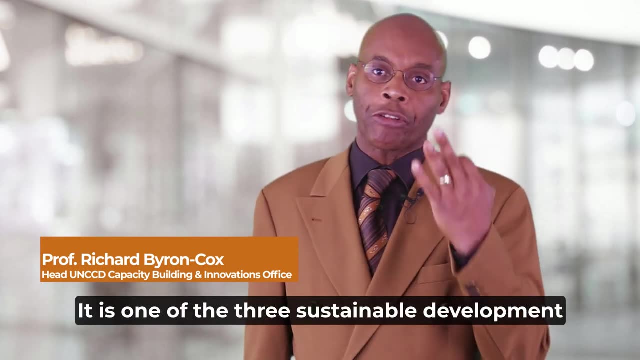 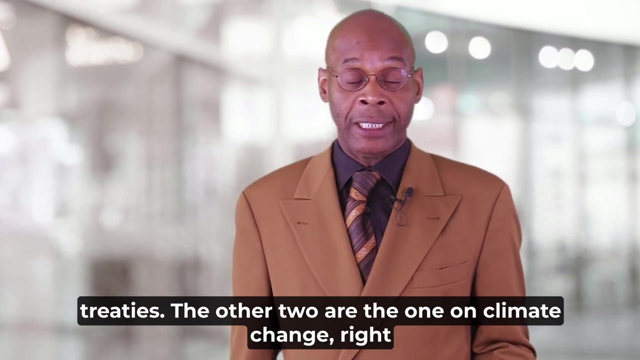 is the UNCCD and what does the CDIO do? Well, the UNCCD is the United Nations Convention to Combat Desertification. It is one of the three sustainable development treaties. The other two are the one on climate change right and the other on biological diversity. More. 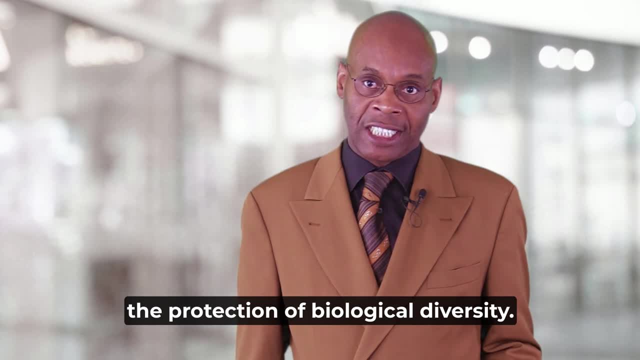 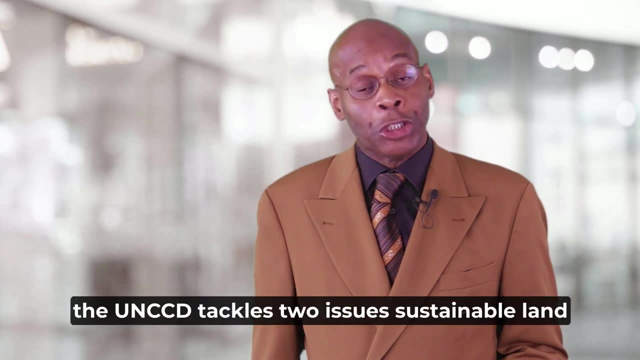 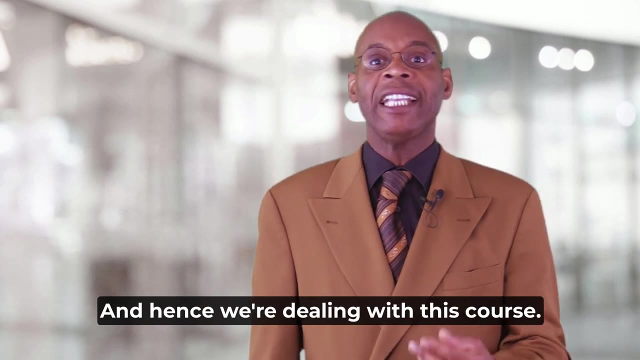 precisely the protection of biological diversity. These three conventions are what we know as the real conventions, which deals with sustainable development. Now, the UNCCD tackles two issues: sustainable land management and the question of drought, And hence we're dealing with this course. My office, the CDIO, is offering this course. 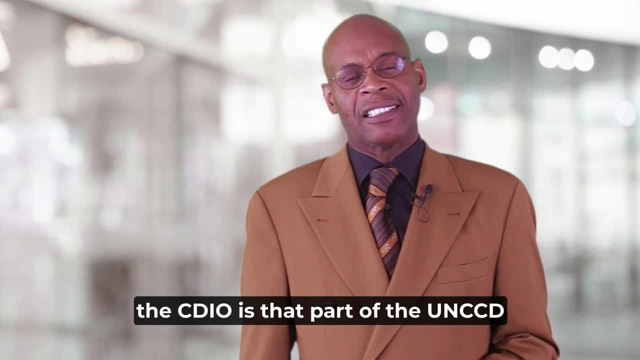 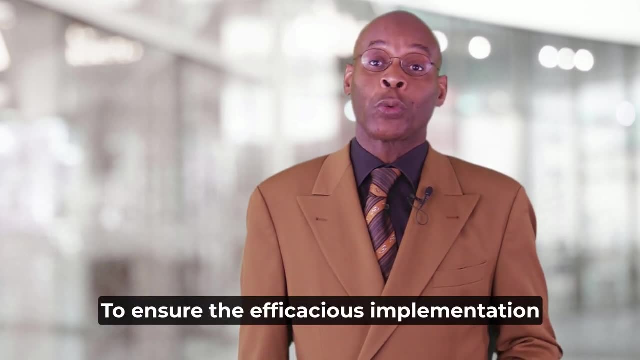 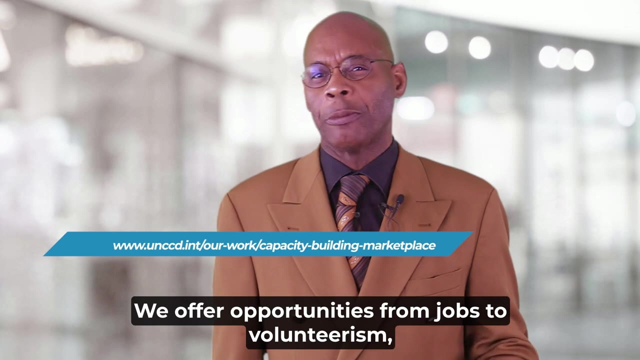 on drought. But what is the CDIO? Well, the CDIO is that part of the UNCCD that deals with capacity development and innovations to ensure the efficacious implementation of the convention. We offer opportunities, from jobs to volunteerism, to scholarships. We offer all of these things. 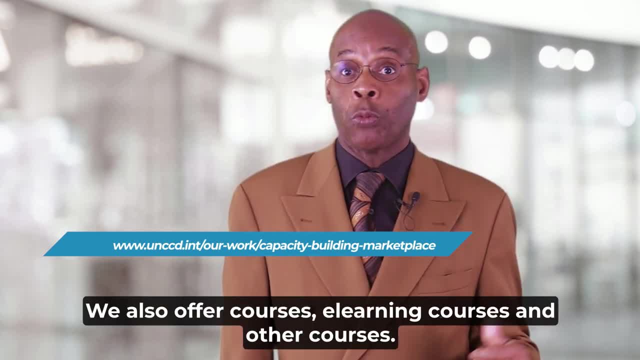 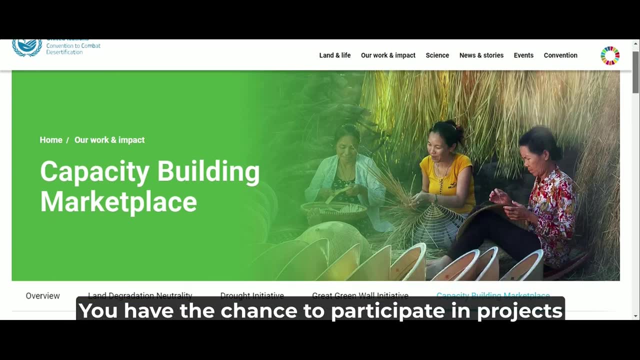 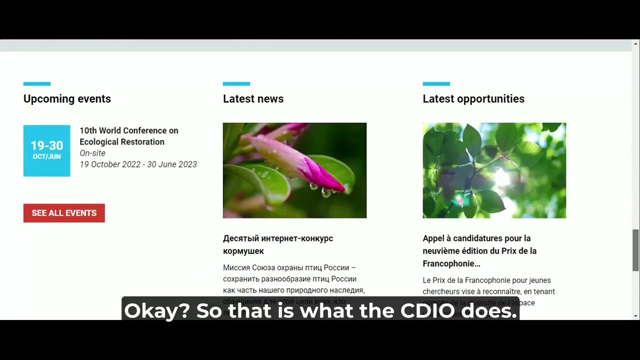 at our website, which you can see Now. we also offer courses, e-learning courses and other courses. You have the chance to participate in projects and we offer an excellent, an excellent internship program. But we do many things okay, So that is what the CDIO does. 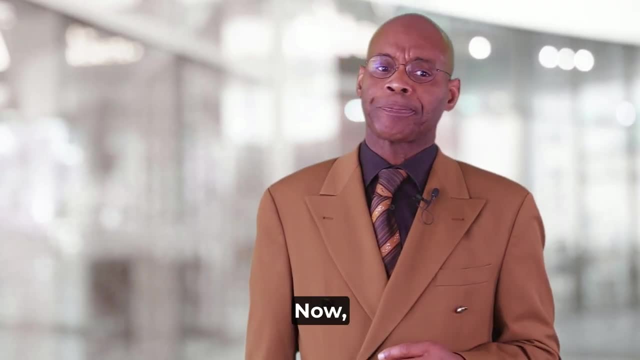 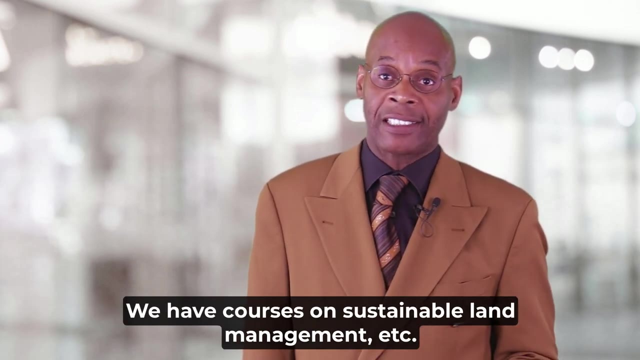 And this is why we are responsible for this course. Now, why a course on drought? Well, we have many other courses. We have courses on sustainable land management, et cetera, But the course on drought, because drought is everybody's. 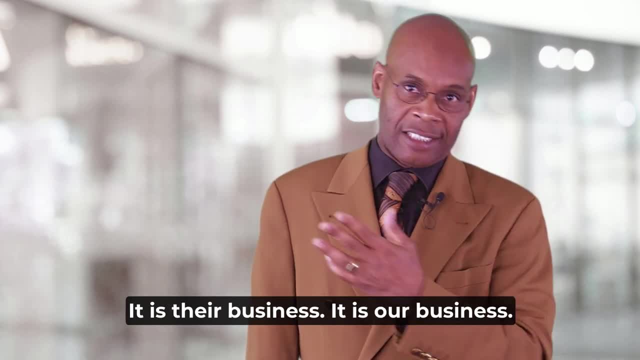 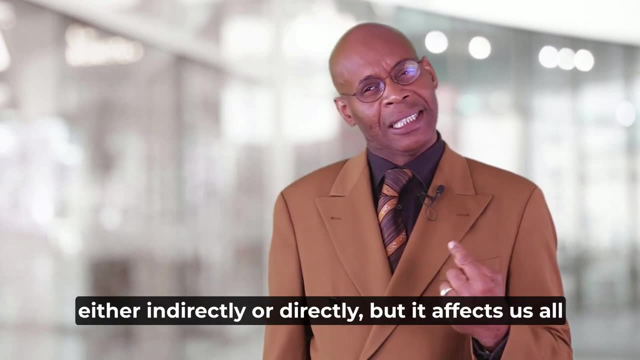 business, It is your business, It is my business, It is their business, It is our business. Why do I say that? Well, because drought affects us all, either indirectly or directly, but it affects us all, And this we will address. 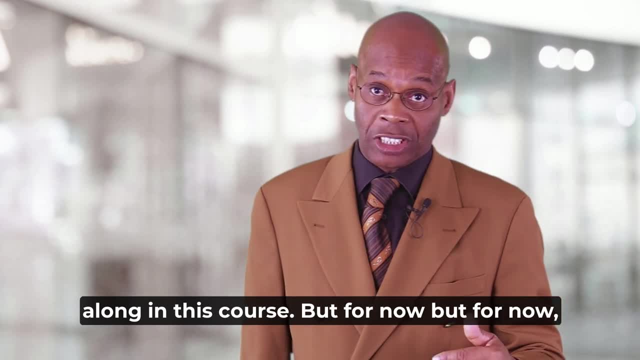 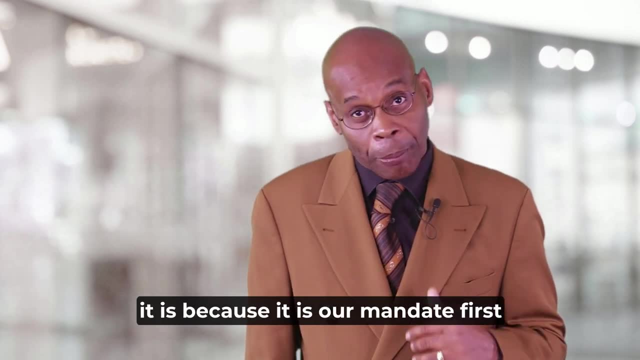 Thank you. We will demonstrate to you as we go along in this course, But for now, but for now, the main reason why we are having this course, it is because it is our mandate, first and foremost, and secondly, because you cannot, we cannot achieve sustainable development. 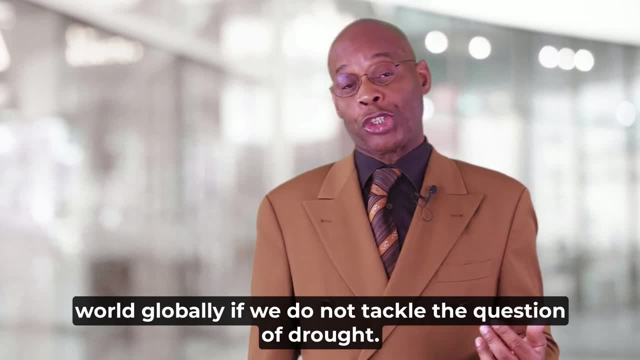 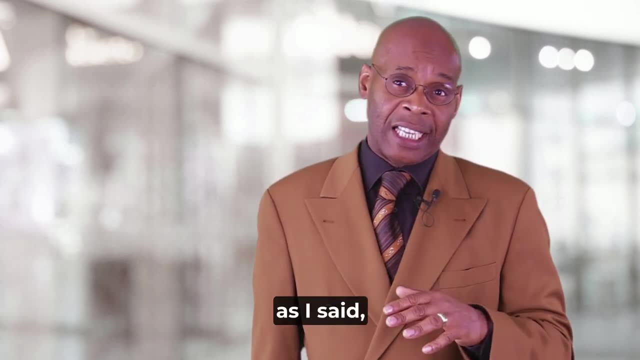 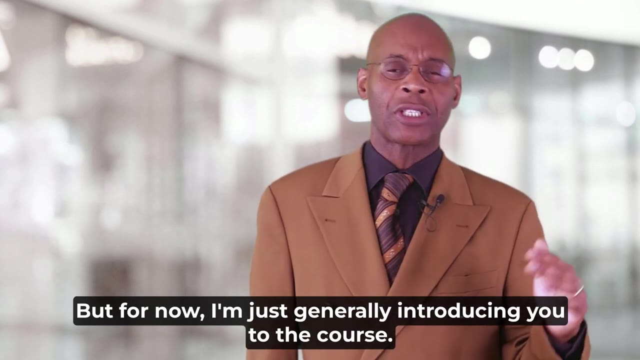 in this world, globally, if we do not tackle the question of drought. We have to tackle the question. This is why we are having this course Now. as I said, we will be telling you more about drought. In fact, a lot of dre- what facing difficulties, but really we will be talking about drought. 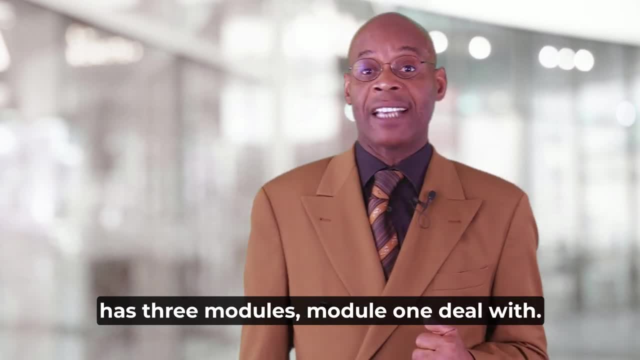 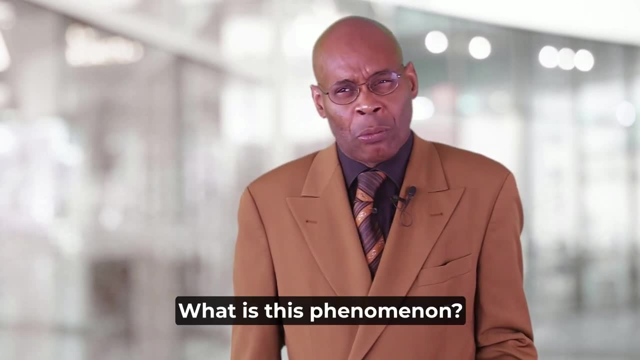 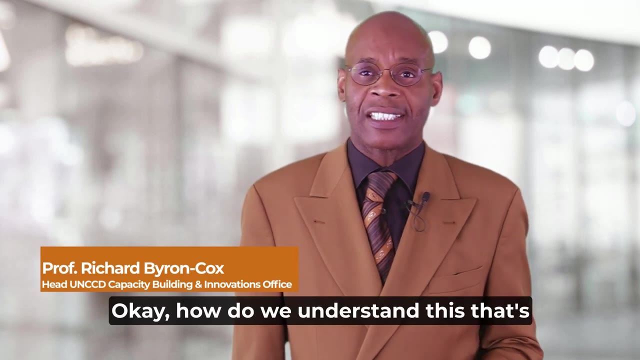 as we go along, But for now I'm just generally introducing you to the course. So what is the structure of this course? Well, it has three modules. Module 1 deals with the question of what are droughts, What is like? what is this phenomenon? Phenomenon, sorry. What does it mean? Okay, How do we? 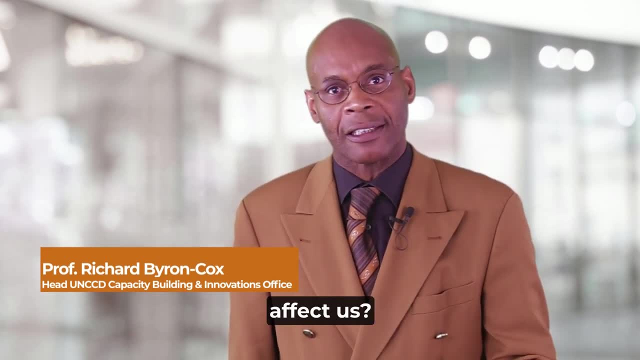 understand this Measure. what, Mister Drought? what is this phenomenon? Phenomenon, Sorry. What does it mean? Okay, How do we understand this? That is module one. Module two deals with the question: does it affect us? In what ways does this drought business affect us? And module three deals with 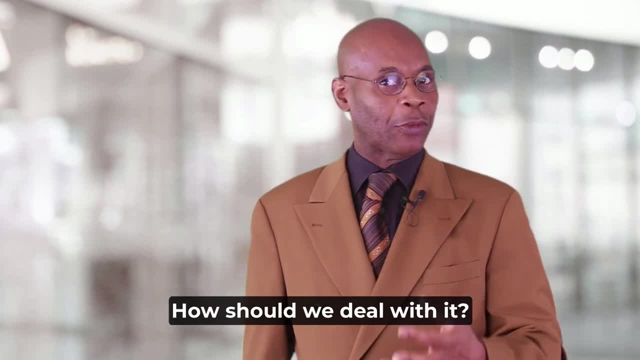 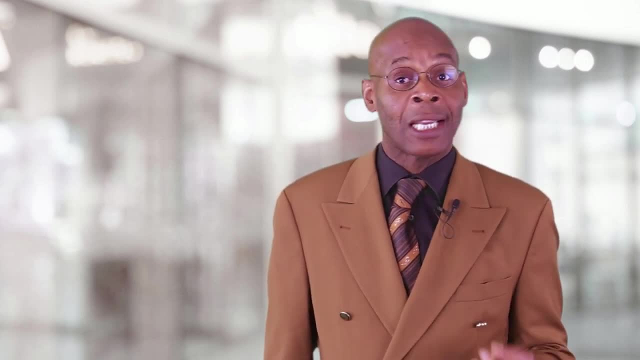 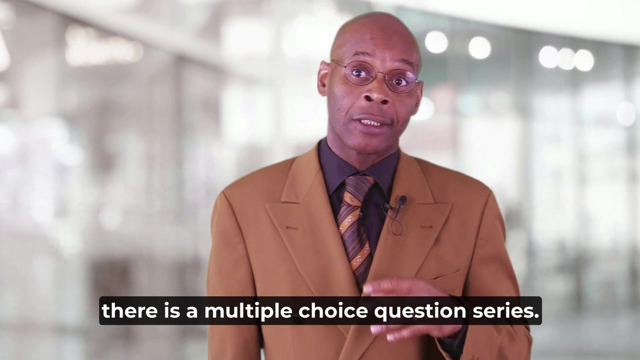 how should we respond? How should we deal with it? In other words, how can we better prepare ourselves to deal with droughts when they come along? So those are the three modules. At the end of the third module there is a multiple choice question series. It contains 30 questions. They're rather 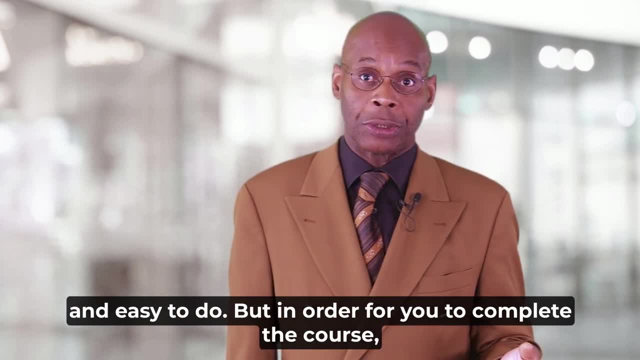 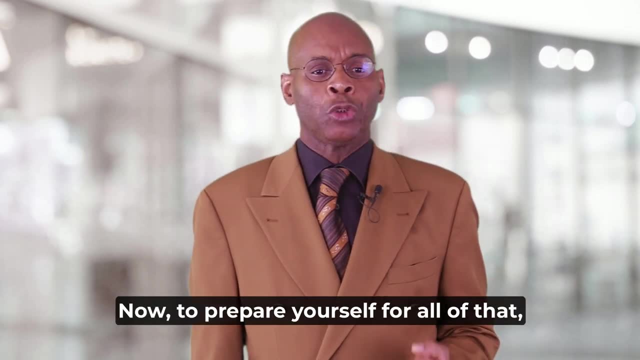 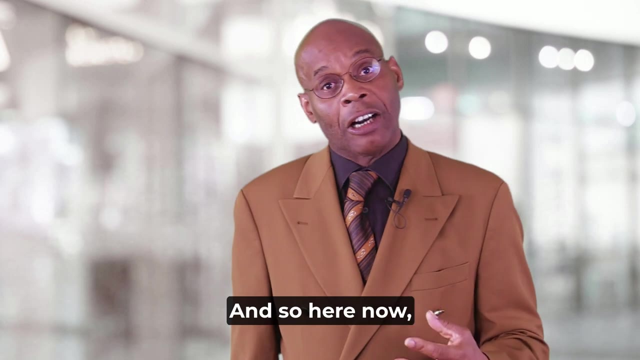 simple, right and easy to do, But in order for you to complete the course, you must take this quiz, this multiple choice quiz, Now to prepare yourself for all of that. of course, right, you have to do certain things, And so here now, I want to give you some general guidance. 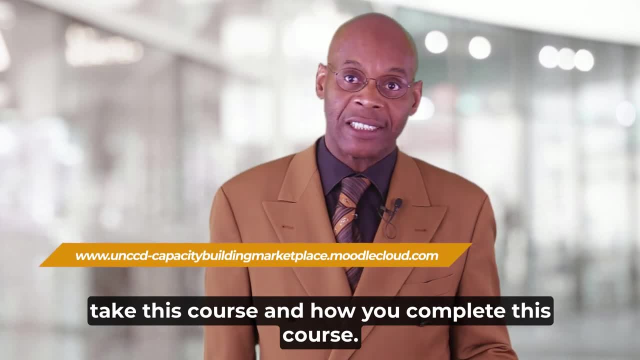 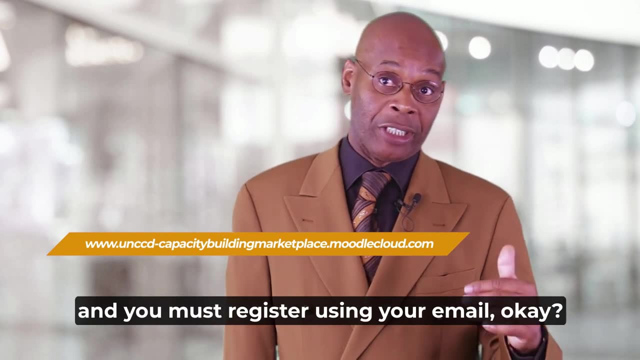 as to how you take this course and how you complete this course. Firstly, you have to register at this site, right, which then gives you access to the course, And you must register using your email, okay? Secondly, in order for you to do the course properly, 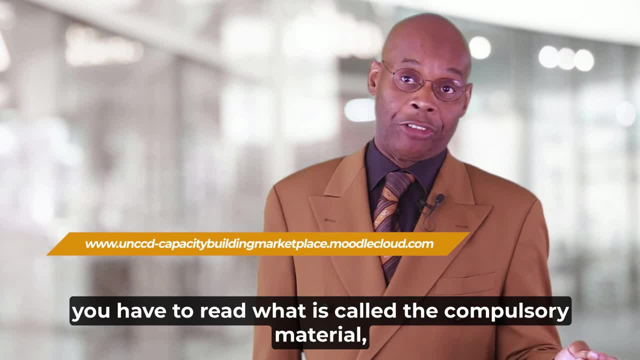 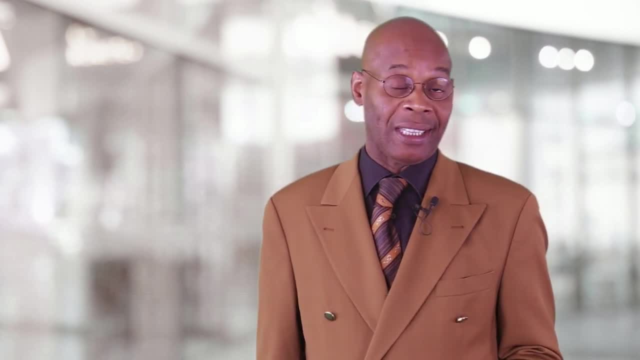 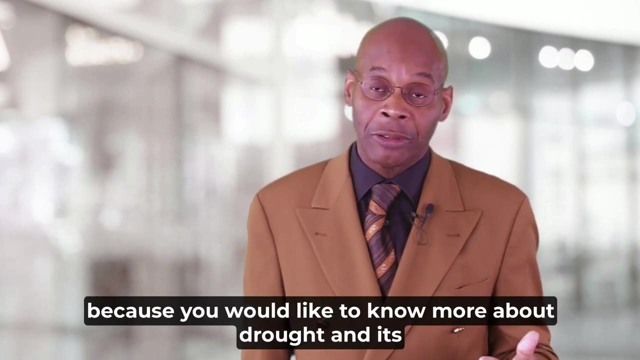 you have to read what is called the compulsory material, In other words, material which you must know in order for you to successfully complete the course. There is additional material you can read if you so wish, because you would like to know more about drought and its effects and its 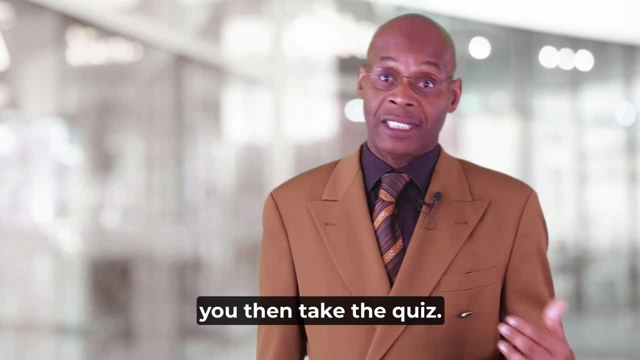 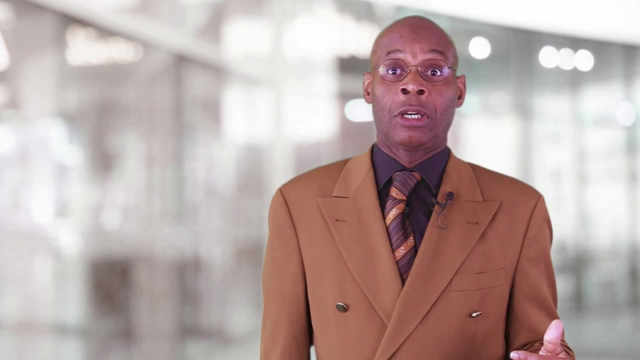 consequences. Then, once you have done that, you then take the quiz. As I mentioned earlier, you must complete the quiz. Once you have completed the quiz, you then make your submission. Now, while you're doing all of that, while you're reading the material, while you're 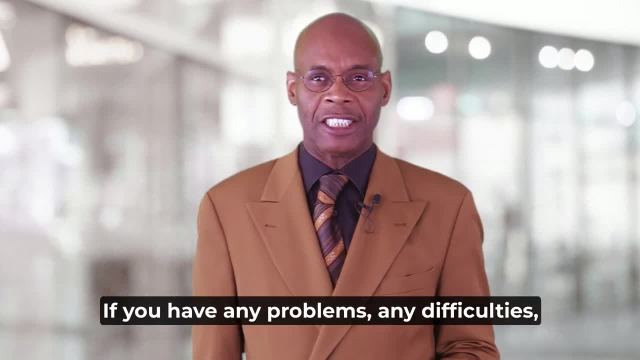 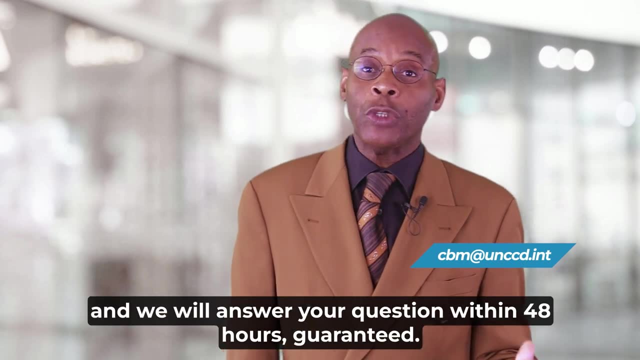 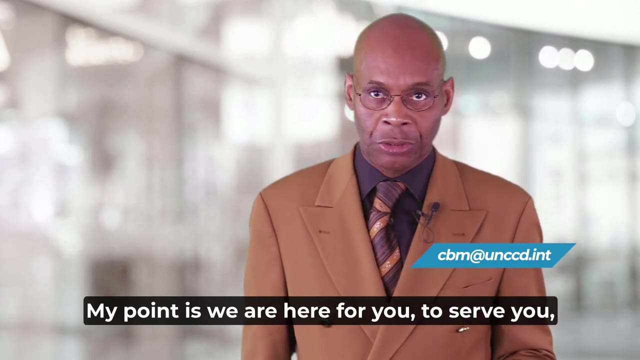 taking the quiz and so on. if you have any problems, any difficulties, we are just one phone call or one email message away. You just send an email to this address and we will answer your question within 48 hours guaranteed. My point is: we are here for you, to serve you. 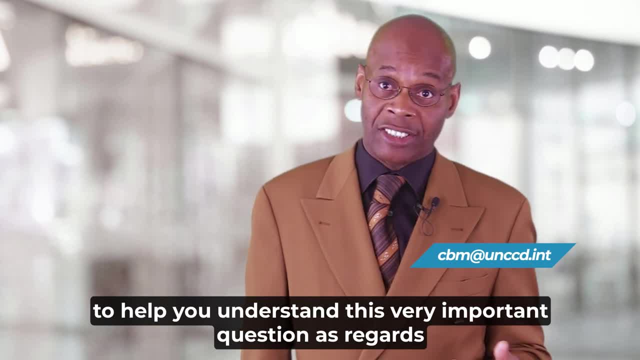 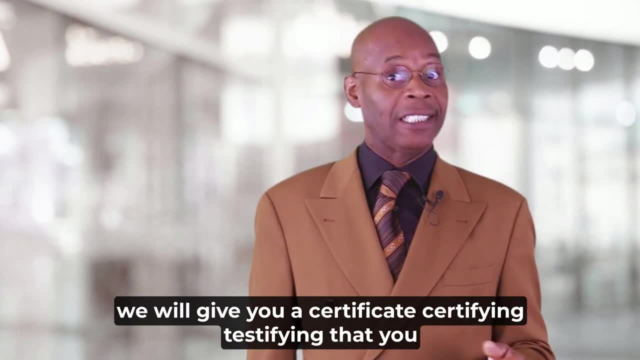 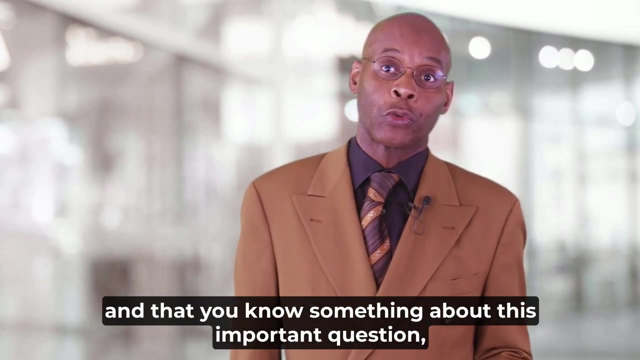 to help you understand this very important question as regards drought. okay, Now, once you have done all of that, we will give you a certificate certifying, testifying that you have successfully completed this course on drought and that you know something about this important question. 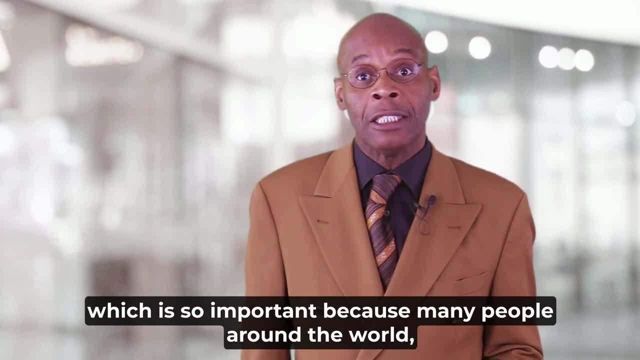 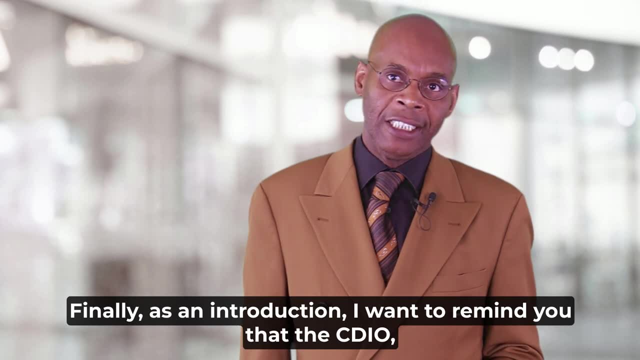 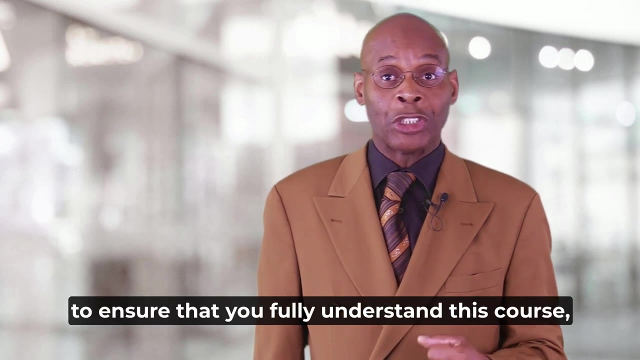 which is so important because many people around the world- most of us- suffer from drought either directly or indirectly. Finally, as an introduction, I want to remind you that the CIO, we are here to support you, to ensure that you fully. 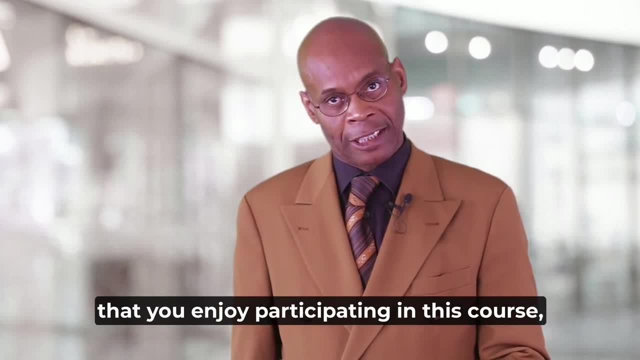 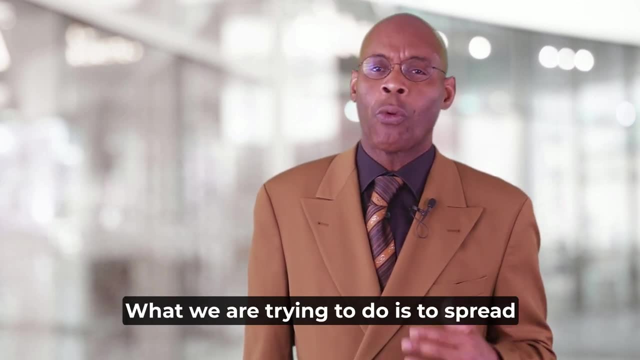 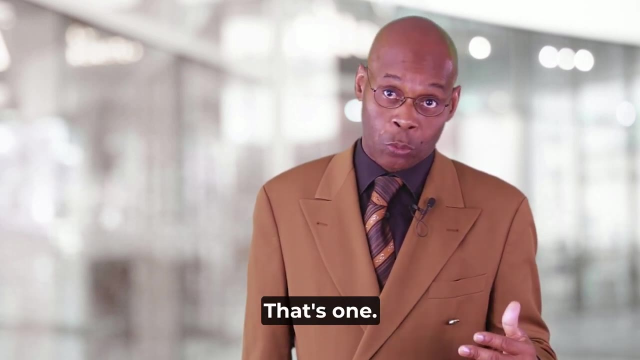 understand this course, that you enjoy participating in this course and that you learn something. The thing is not to test how brilliant or how talented you are. That is not the issue at all. What we are trying to do is to spread the message that drought impacts us all. That's one. 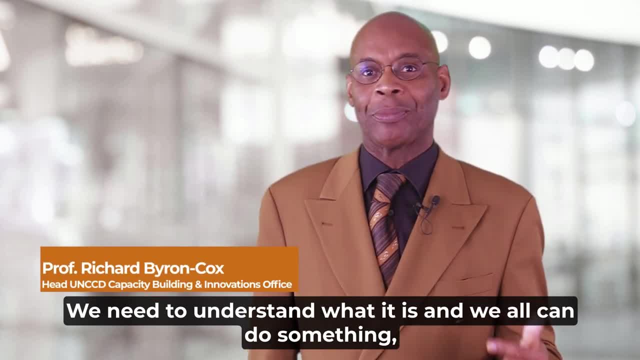 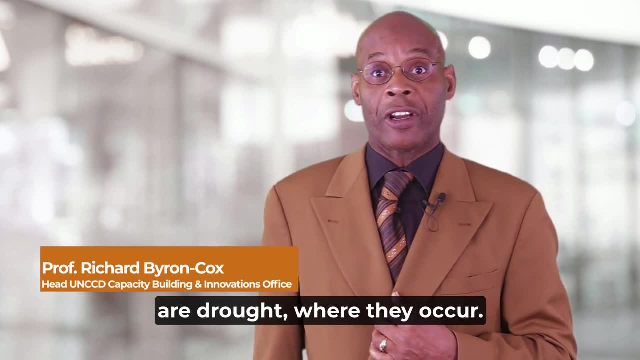 We need to understand what it is and we all can do something you understand and we can prepare ourselves to better handle drought. The next lecture we will get directly into water droughts where they occur. Until then, I'm Richard Byron Cox. See you next time.